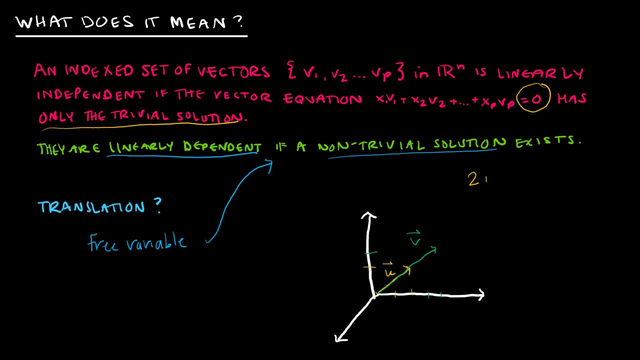 just as easily have taken 2 times vector u to get to this exact same place that vector v ended up, which is at 4: 2.. So if you have a situation where one vector is the multiple of another, then they are linearly dependent. If I were to have, say, vector w, that's out here at 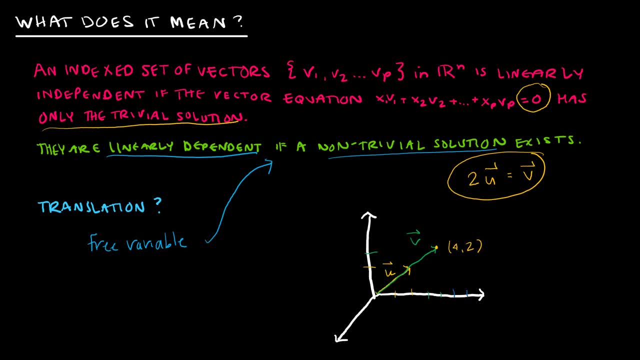 6: 1. Maybe I should do a better job there. So this is vector w. Now, clearly I can't just take some multiple of u or some multiple of v to end up at vector w. so vector w would be independent of vectors u and v. Let's take a look at a practical question. 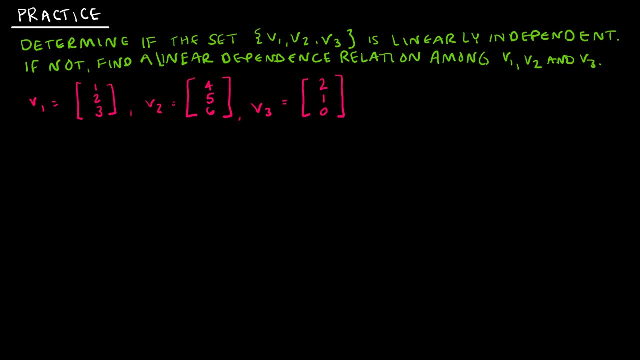 What is the illustration of vector v? Let's take a look at a practical question. What is the illustration of vector v? Let's take a look at a practical question question together. The question itself asks us to determine if the set of vectors V1,, V2, V3 is linearly independent and, if not, to find the linear. 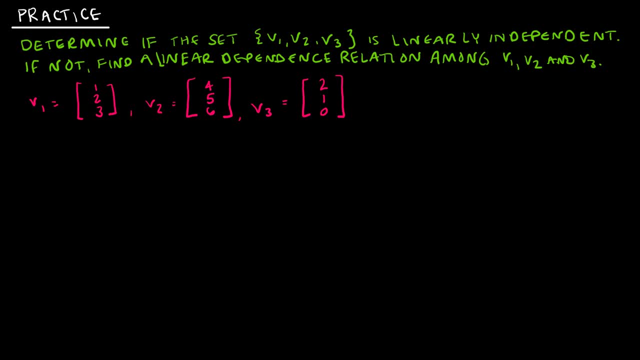 dependence relation among V1,, V2, and V3.. So this might look like a brand new question that we've never tried to answer before, but really we already know exactly what we're doing. All I'm going to do is I'm going to take these vectors. 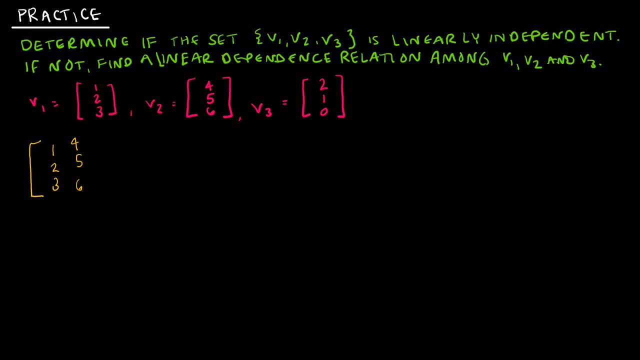 and I'm going to create a matrix and I'm going to put them on a matrix and I'm going to use a matrix and I'm going to call this matrix by matrix and matrix, And this is essentially what I'm solving. Remember we're looking at: does the matrix equation equal zero or the vector? 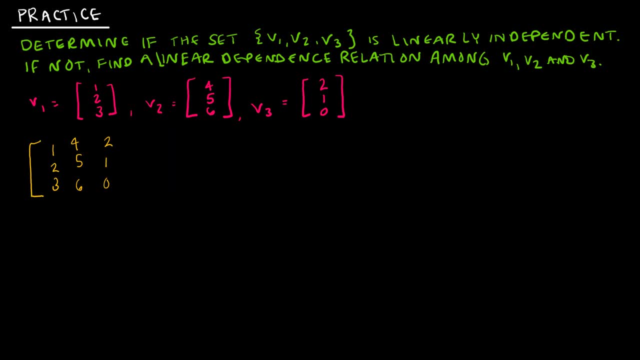 equation equals zero, and so I can do this augmented matrix with the column of zeros. but remember, when you're dealing with a homogeneous system, that last column is always going to be zeros. So it's still okay for me to just focus on the coefficient matrix. So I'm just going to stick with this matrix and 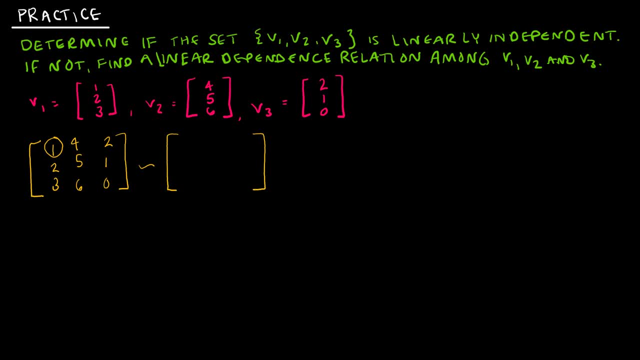 columns and pivot positions and I'm turning everything above or below that into zero. so this will be one four two. I'll take negative two times that first row plus the second row, and that's going to give me a zero right where I want it, and then negative three and negative three. then I'm going to take negative. 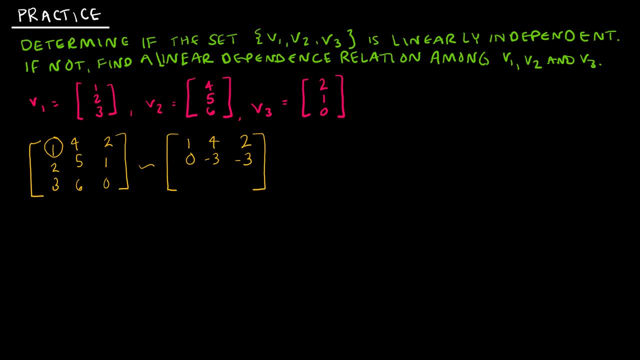 three times the first row and add it to the third row and that's going to give me zero and negative six and negative six. then I'm going to continue. I'm going to keep my one, four, two, that second row. I'm going to divide everything by. 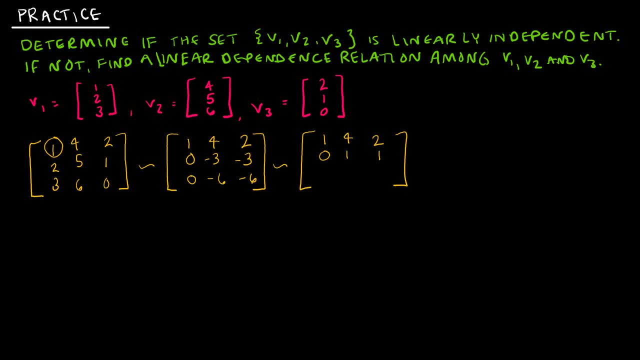 negative three and the third row, I'm going to take negative two times the second row and add it, and that gives me zero, zero, zero. so if this question just said determine if the set of vectors is linearly independent, I could stop right here, because I've got a set of vectors that are linearly independent and I 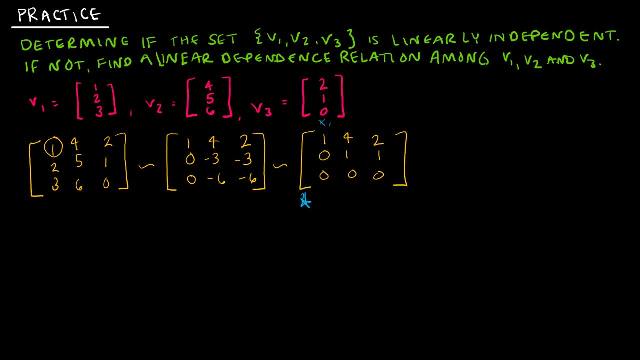 just answered the question. remember, this is x1, this is x2 and this is x3. x1 has a pivot, x2 has a pivot, x3 no pivot, which means x3 is free. so what does that tell us? that tells us there's going to be non-trivial solutions and that means the 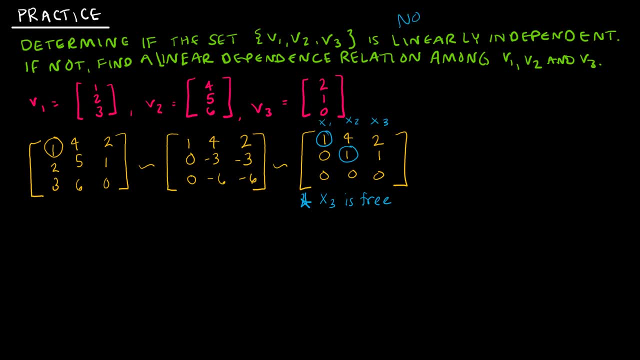 answer is no. they are not linearly independent. they are linearly dependent. now we are asked to continue. it says: if not find the linear dependence relation. so what do they mean by that? all they're saying is: keep up your good work here. so I'm going to take that second row. well, 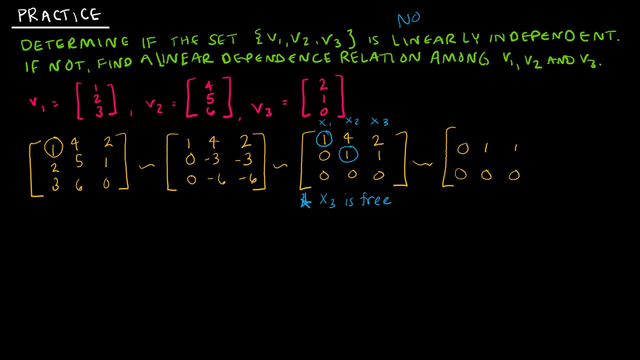 let me just go ahead and rewrite these. I'm going to take that second row times negative 4 and add it to my first row. so negative 4 times 0 plus 1, negative 4 times 1 plus 4 and then negative 4 times. 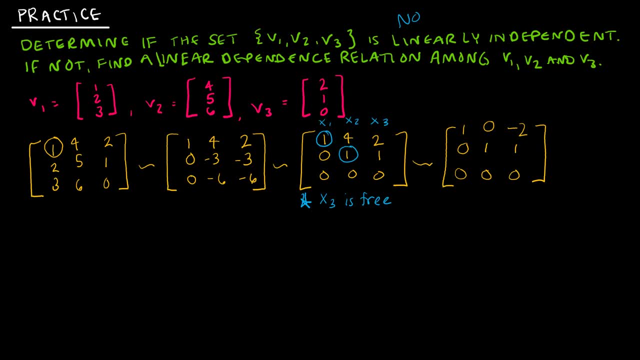 1 plus 2, and that gives me this situation here. so what does that tell me? well then, x2 is equal to 0, and I always rewrite that as X 1 is equal to 2, X 3. well, remember that this says X 1 minus 2, X 3 is equal to 0, and I always rewrite: 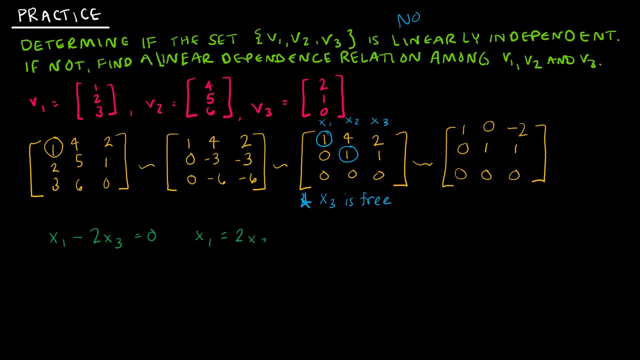 that, as X 1 is equal to 2x 3, and then X 2 plus X 3- whoops plus X 3 is equal to 0 and of course, 3 plus 1 equals 0 and that's not going to change. and so D is equal to 2X 3 is equal to 0 and of course we- your override- could be the key to your override. 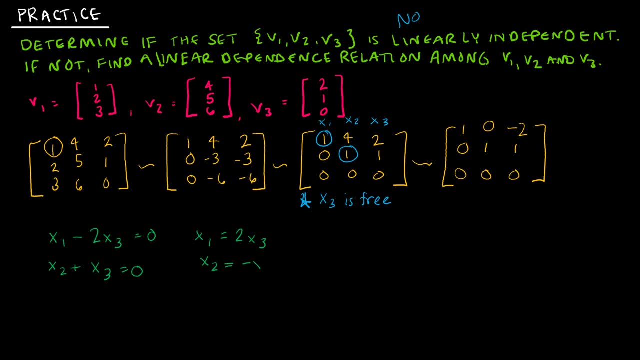 course, we always wrote that, as X2 equals negative X3. And then X3 is free, And so that is our solution, And we can leave it exactly like this. So if we're looking for some sort of relation, we can just basically make up a value for X3. So let's let X3 equal 2.. 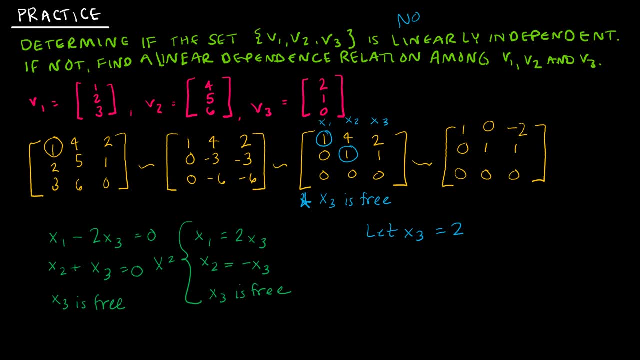 Well, what is that going to do? That's going to make up a value for X3.. So that's going to be: X1 is going to be 2 times X3, which is 4.. And then X2 would be negative, X3,, which is negative, 2. And X3 would be 2.. 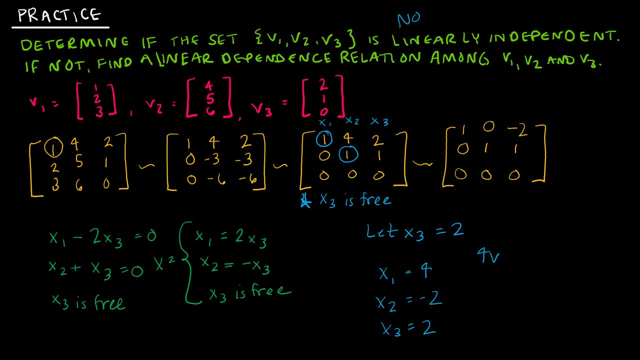 So what is that going to look like? It's going to be 4V1 minus 2V2 plus 2V3 equals 0.. So that is one out of however many, infinitely many, because obviously I can make up whatever. 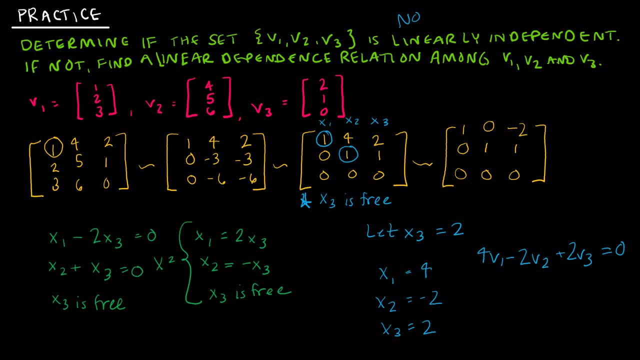 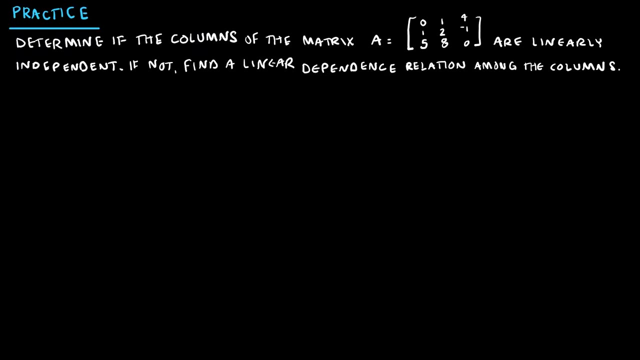 value, I feel like for X3, possible linear dependence relations. So essentially all we're doing is exactly what we were doing before, And then I can substitute a value in for my free variable. Here's a practice for you to try on your own. So if you would press pause, try this. 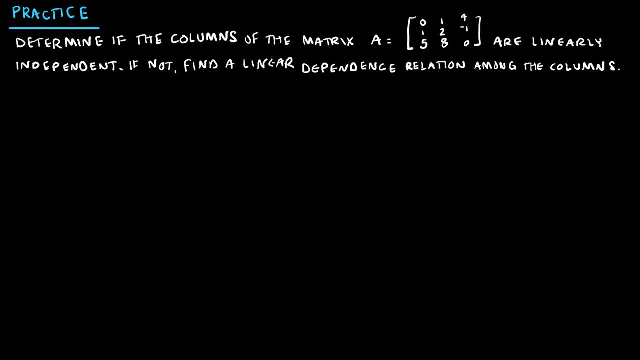 question. When you're all done, press play to see how you did. Here we already have matrix A, And again that's just made up of three different vectors. So this question is exactly like the last question. They've just already done that first step for us. 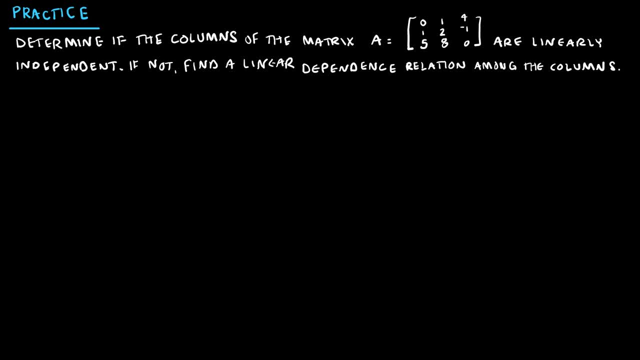 by taking the vectors and putting them into a matrix. So we can take that matrix: 0, 1, 5, 1, 2,, 8, 4, negative: 1, 0.. And remember, it's okay to have this last column, because that's what we're looking at is an augmented matrix On. 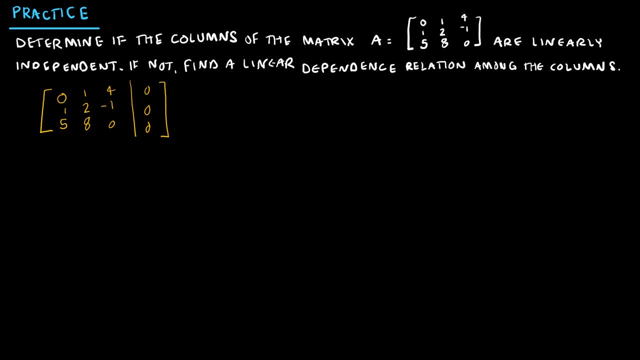 the last example. I didn't put that 0 column in there This time. I'm going to leave it there. It's correct either way. So what I'm going to do is just as I have been doing. I'm going to do my row. 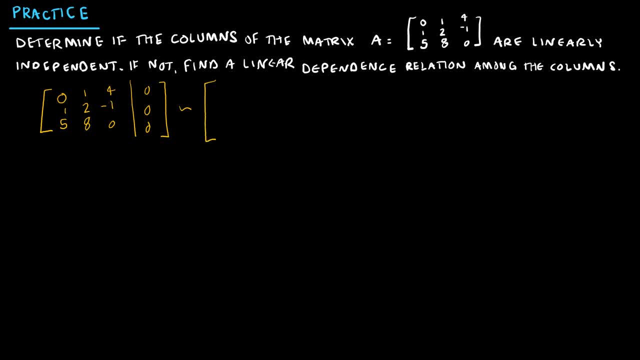 operations. Now this one. the first thing I'm going to do is notice I've got a 0 right here where I'd really like to have a pivot, So I'm actually going to interchange those two rows. I'm going to make this 1, 2, negative 1.. 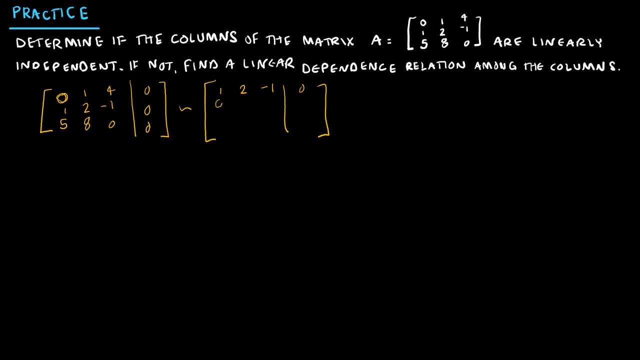 And then I'm going to move this row down, so that's 0, 1,, 4, 0.. And I already have a 0 now in that second column where I want it. I want a 0 in that last column, So I'm going to take that. 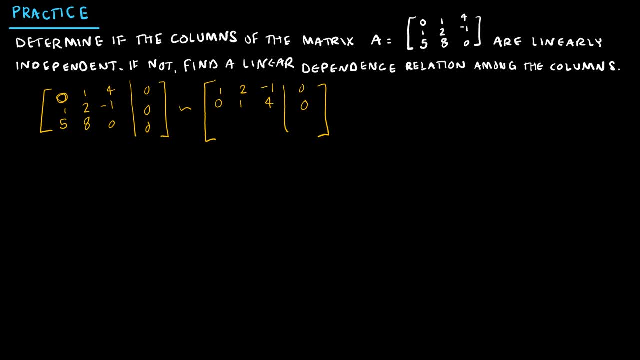 first row, my new first row, which is really my second row- times negative 5 and add it to row 3.. So negative 5 plus 5 is 0.. Negative 10 plus 8 is negative 7.. So 9 plus 10 minus 7 is 19, and 2 on 2 is 19.. 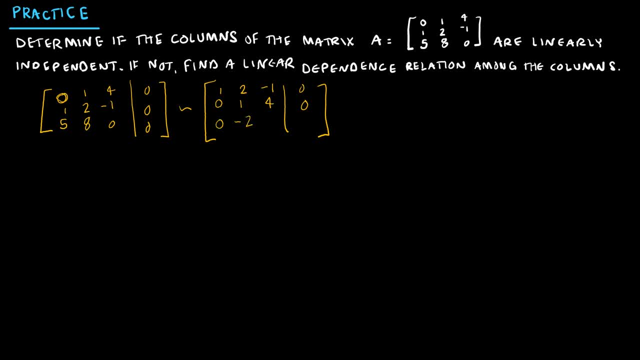 Both things are interesting, I'm pretty sure. So let's re-multiply. this is really how we would 1 the first row down. I'm going to move this: negative 2, positive 5 plus 0 is positive 5, and then 0.. And now I'm going to continue. 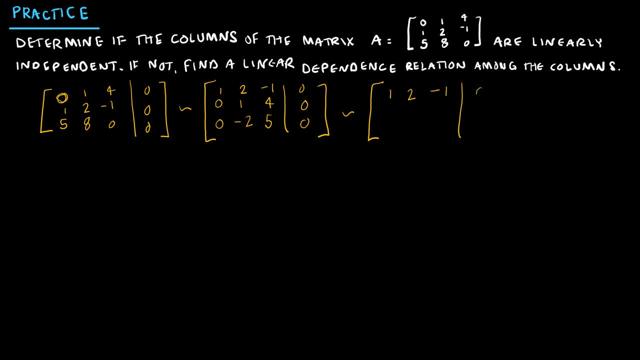 I've got my 1, 2, negative 1, and I'd really like this guy then to be my pivot, And so I need to make that negative 2 into a 0. So if I take that second row times 2 and add it to, 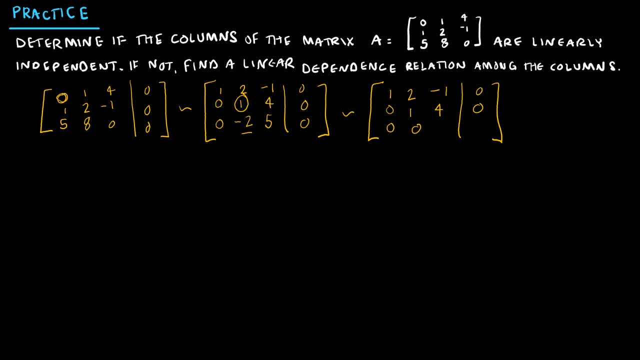 my third row. so I'm going to have 0 here, 0 here, 8 plus 5, that's 13.. And now I'm going to stop right here. So the question says: determine if the columns of the matrix are linearly independent. 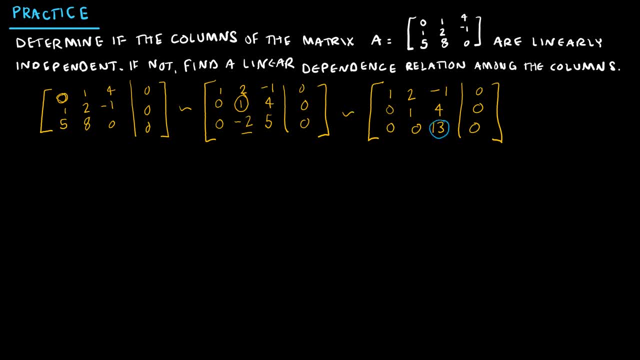 And so what I'm looking at is, obviously, this is not a free variable. There's not 0, 0, 0, 0.. This is a basic variable. This is going to be a basic variable, and this is going to be a basic. 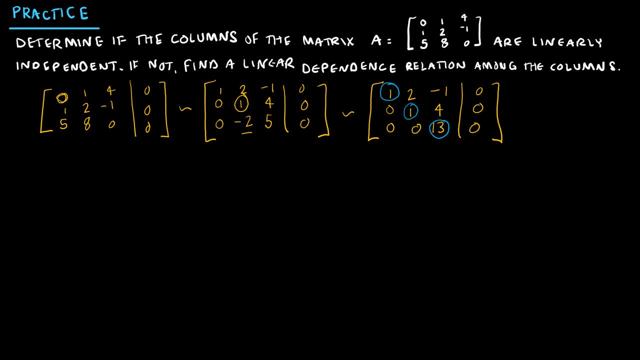 variable because I have pivots in each of the columns. So, since I have three basic variables, there are no free variables, No free variables. So I'm going to take that first row and add it to my column. So I'm going to take that first row and add it to my column. So, since I have three basic variables,